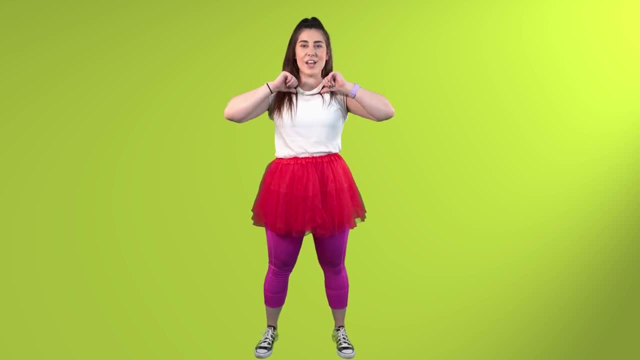 to put our arms back in the air, Wave them around, Point to yourself, Show me your muscles And then show me your roar again. And then we're going to do some little roars while she's singing, Alright, ready to take it from the top. Alright, Point Roar All the way to the other side. Hands in the. 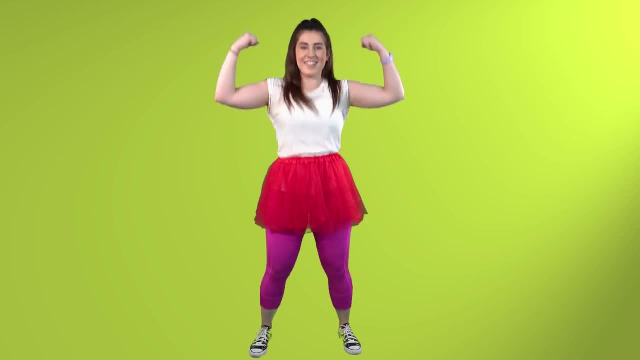 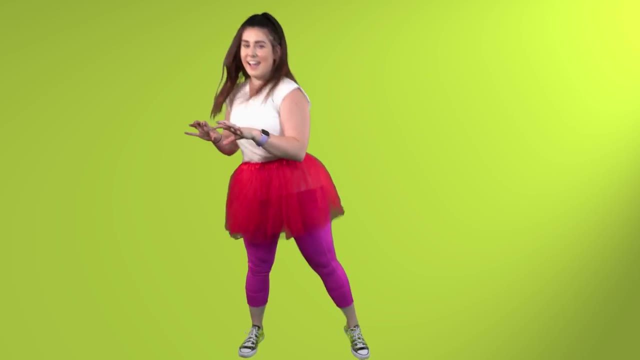 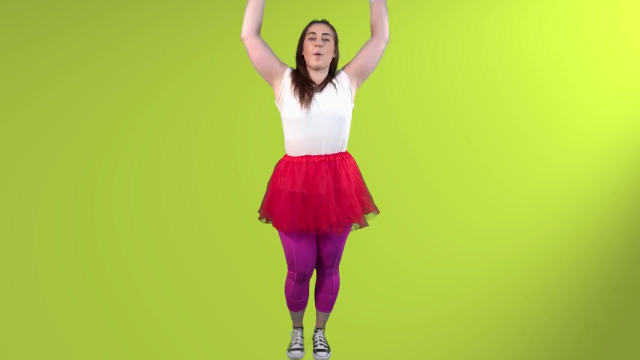 air. Show me your muscles- Good Hands in the air. And show me your muscles again Good. And then roar. And then the little roar- Awesome, Good job. Alright, let's take it from the top. Good job. After that, we're going to do some spins as a butterfly, So show me your. 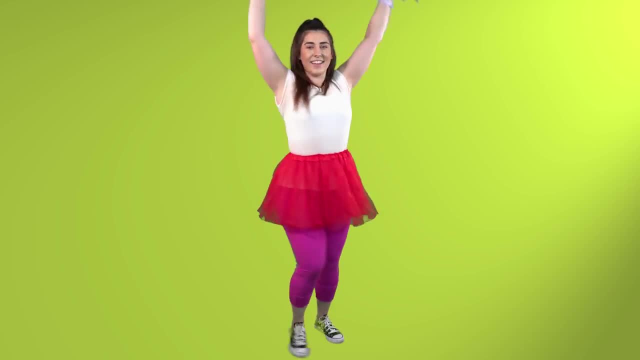 big, long butterfly wings and we're going to go in some circles And you're going to keep going around And then she's going to say zero. So you're going to show me your zero And then you're going to show me a superhero pose. You can stand on one foot, lean up and 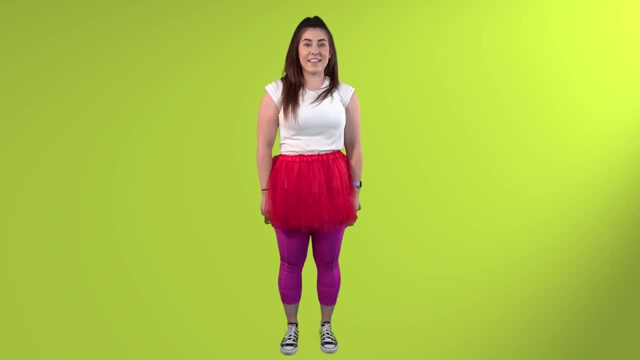 kick your other leg out- Good job. So let's try that again, Ready? So show me your butterflies going in circles- Beautiful, Good job. Alright, jump out. Show me your zero- Good job, Good job. And then show me your superhero. And then show me your superhero- Good job After that. 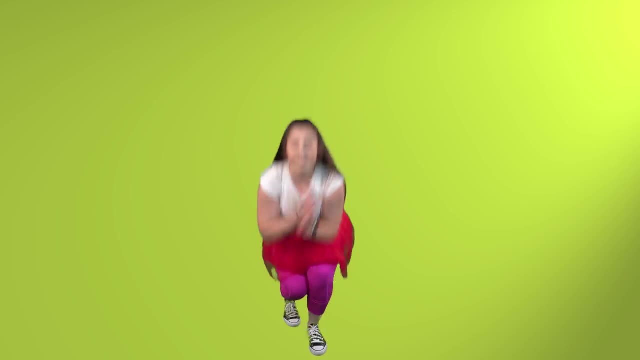 she's going to say: help me down. We're going to bop all the way down and then jump back up into a star. And then, hands in the air- Good. We're going to point to our ears, So like this And hand on your other hip- Good. Hands in the air, Good. And then we're going. 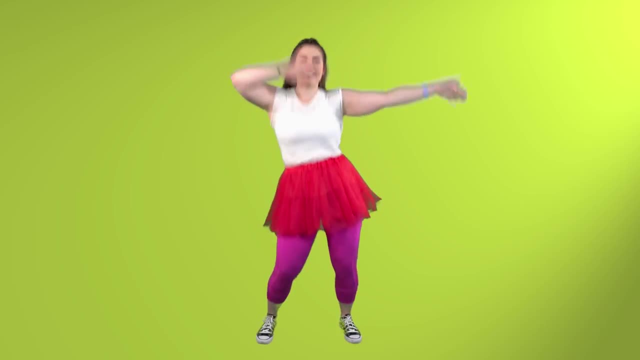 to bop back down again All the way up Hands in the air. Then after that we're going to point to our eye And then we're going to get ready to go again. I got the eye of the tiger All the way around. 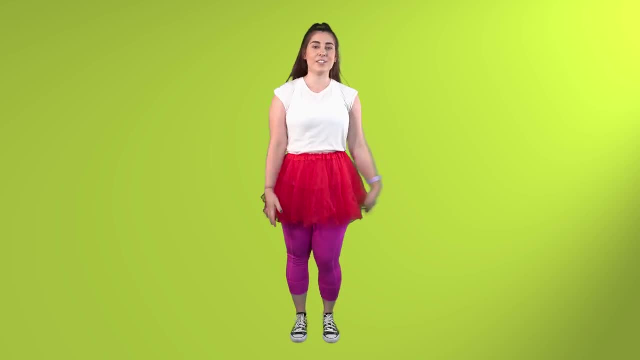 And we repeat the chorus. Let's take it from the top. Ready, A little butterfly In a circle, Beautiful. Show me your zero, Show me your hero. Bop down All the way up, Hands in the air. And then we're going to bop down again. All the way up, Hands in the air. Good, 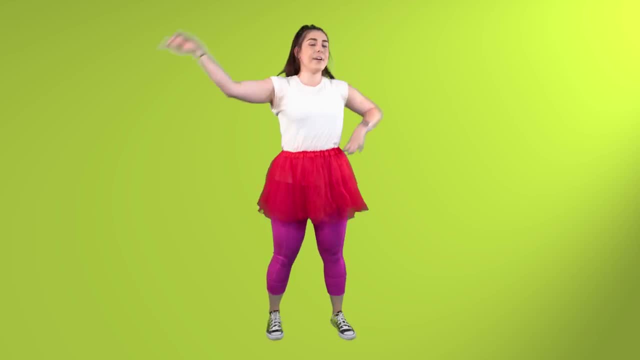 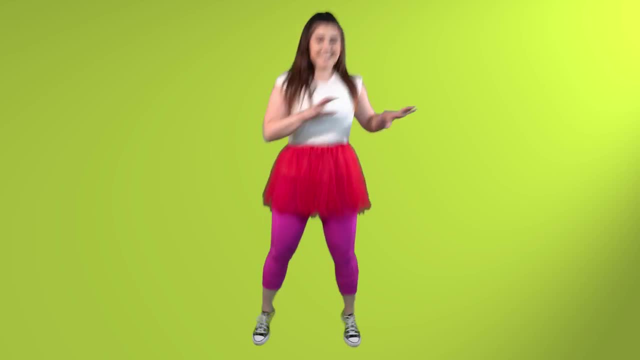 take it all from the top, Ready, Point down down, Hands in the air. Good, Point to yourself: Show me your muscles, Awesome Arms in the air. And then point to yourself, Show me your muscles, And then tiger, tiger, And then your little rose. Okay, now you're going to. 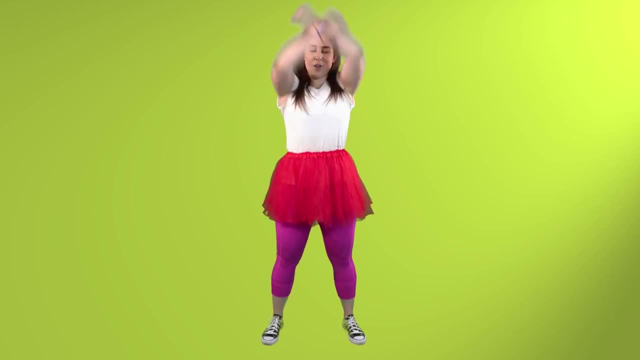 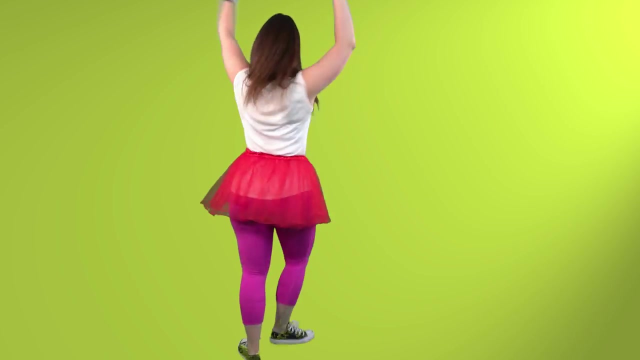 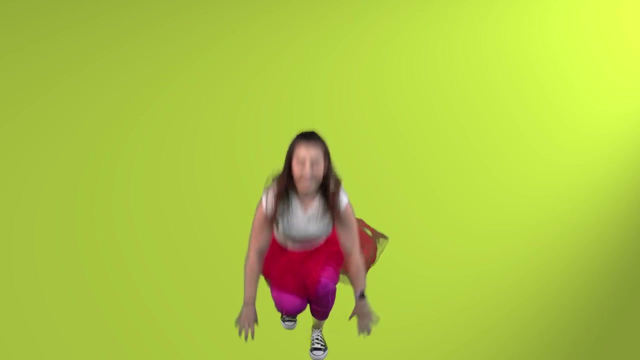 do guys pop? Good, Okay, now 16 of these servers. Great, Awesome, Awesome. So we've got the butterfly. beautiful, show me your zero, show me your hero, and then flop down all the way back up hands in the air. good job, flop back down, hands back. 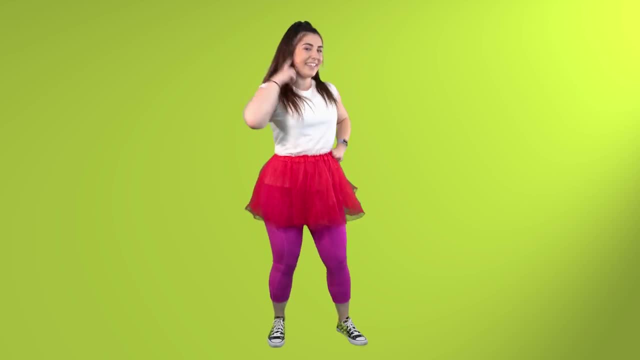 up. good. point to your ear. good hands in the air, point to your eyes, and get ready to go again. good hands in the air, point to yourself. show me your muscles. good, awesome, get ready to roll. good hands back in the air. alright, show me your muscles and then. 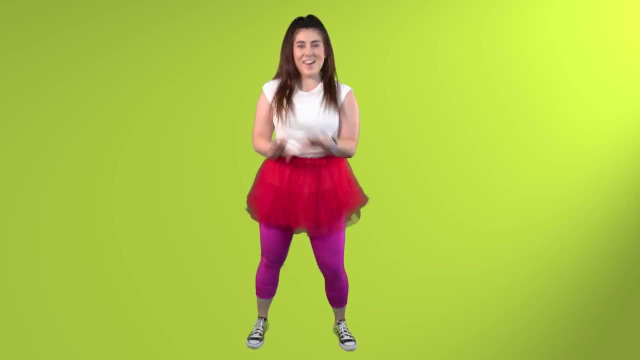 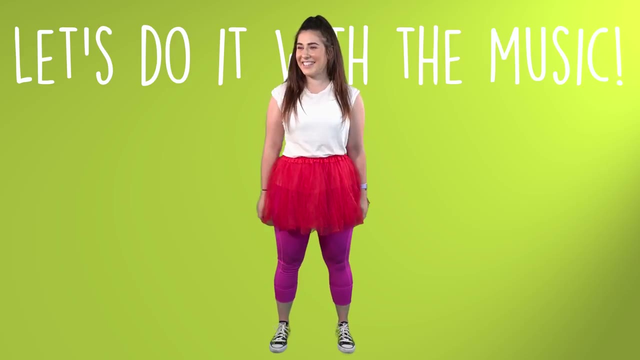 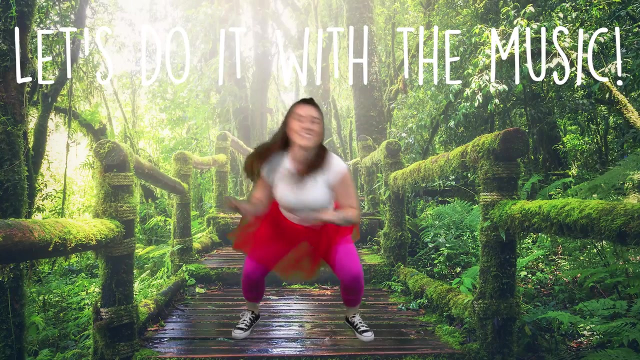 we're going to do our little waltz. good job, awesome, such a good job. ready to do it with the music. Cool, Hit it with some music. I see it all. I see it now. I got the eye of the tiger, the fire, dancing through the. 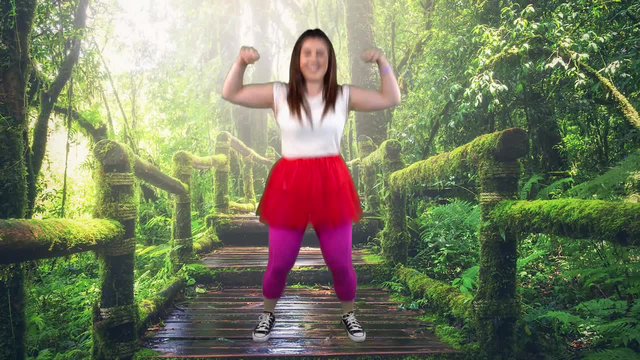 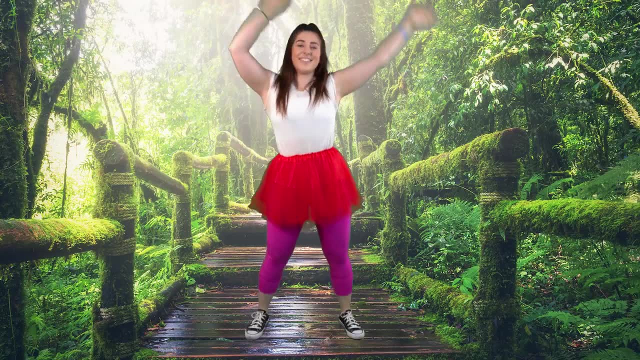 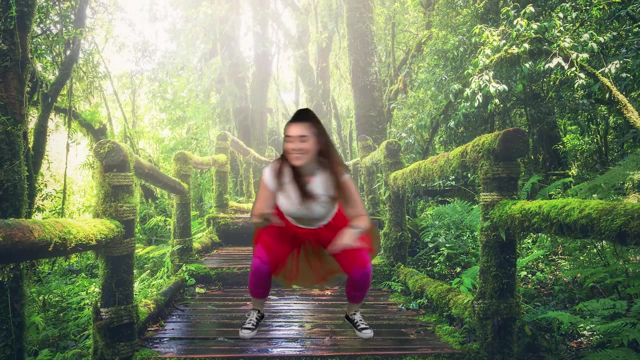 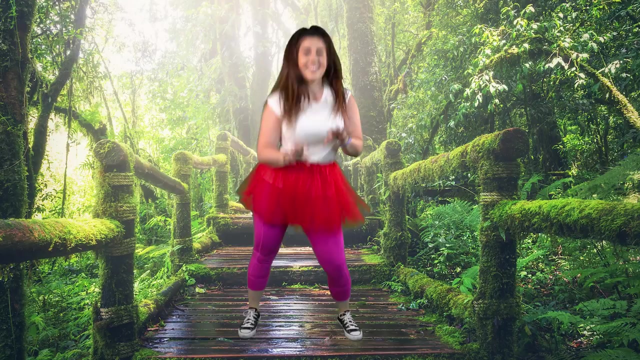 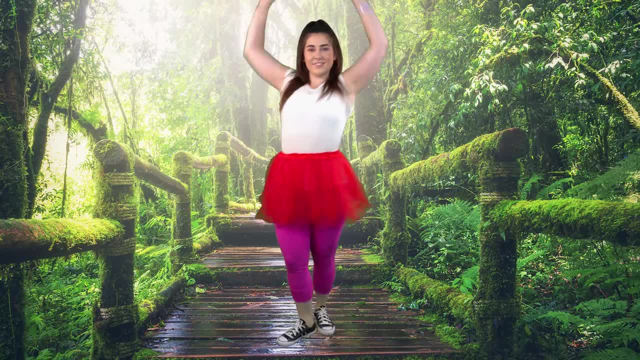 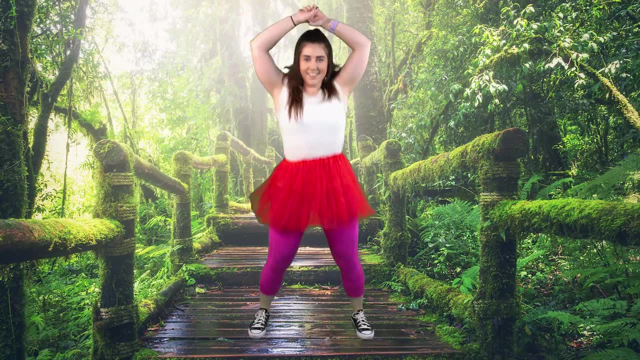 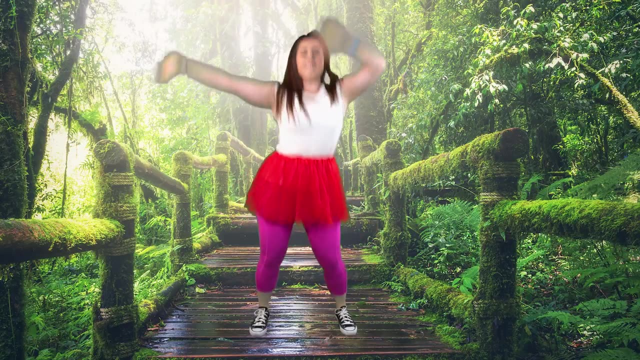 hear me roar. Now I'm floating like a butterfly, stinging like a bee. I earned my stripes. I went from zero to my own hero. you held me down but I got up already brushing off the dust. you hear my voice. you hear that sound? 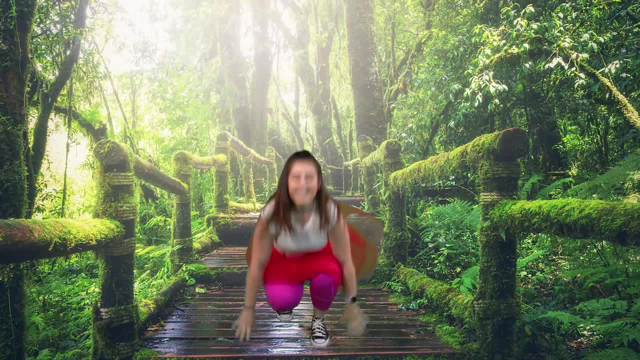